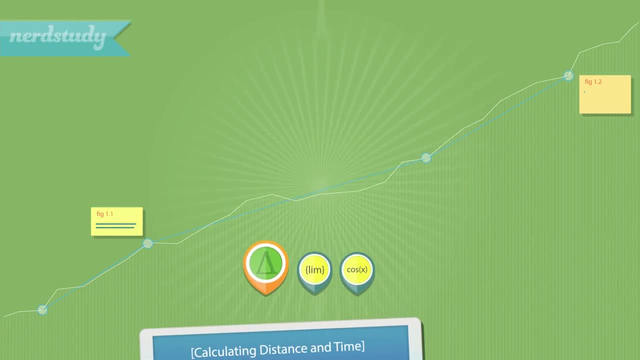 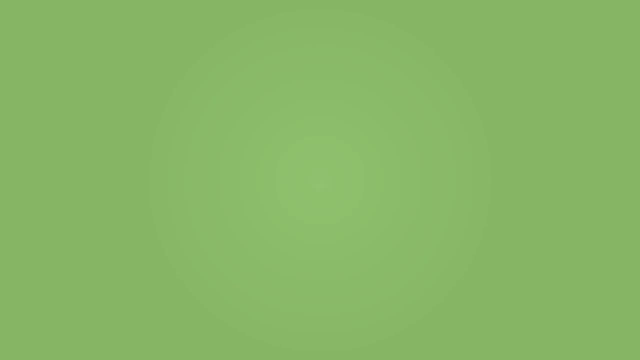 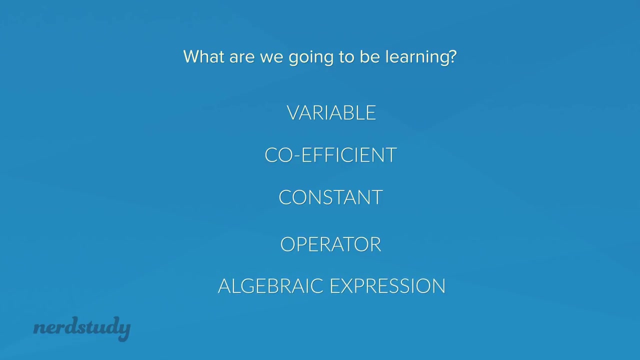 In this video, we're going to learn about variables, coefficients, constants, operators and how to write algebraic expressions. In order to learn some of the new math concepts down the road, it's important that we go through some definitions together. And don't worry, because 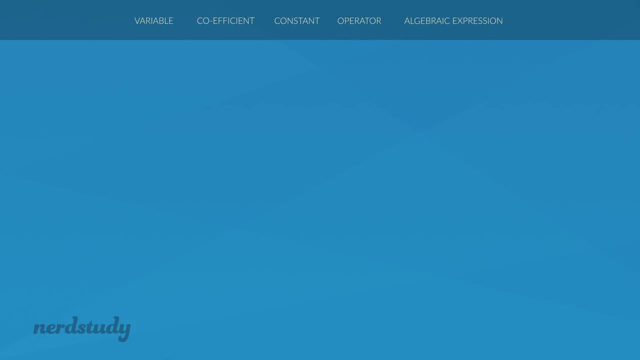 they're really not too difficult to learn. We already know what a variable is. Let's say, there's a variable like d. Well, sometimes you will see a number immediately before a variable like 5d. A number and a variable side by side actually means that they're being. 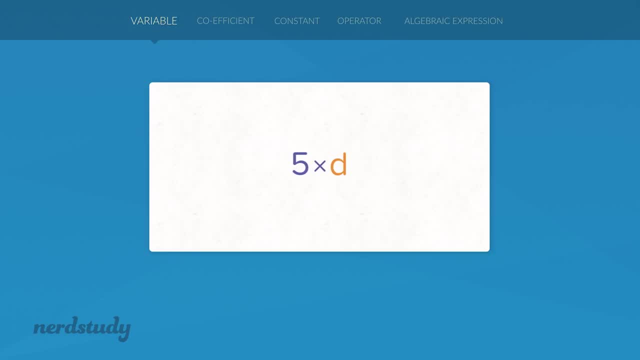 multiplied together. So this just means 5 times d. The 5 over here is called a coefficient. A coefficient is a number that is placed before a variable and is being multiplied with a variable. Be sure not to confuse a coefficient with a constant. A constant- 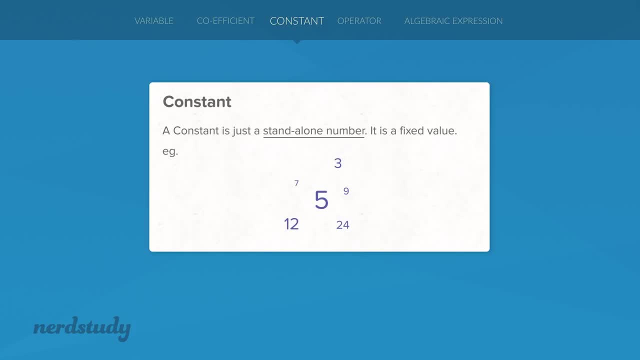 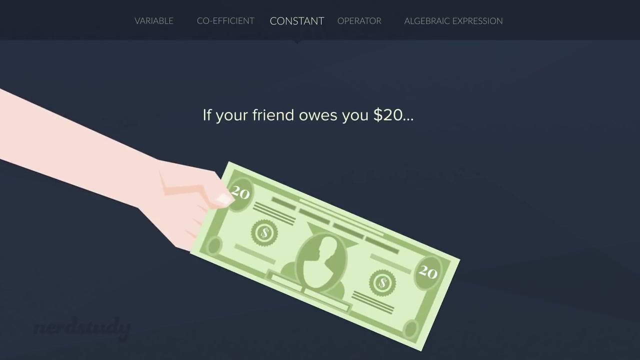 is just a standalone number. It is a fixed value. Since it's not a variable and it's not being multiplied by a variable. the value of a constant does not change. For example, if your friend owes you $20, he literally owes you exactly $20.. You know the amount that he owes you and it won't. 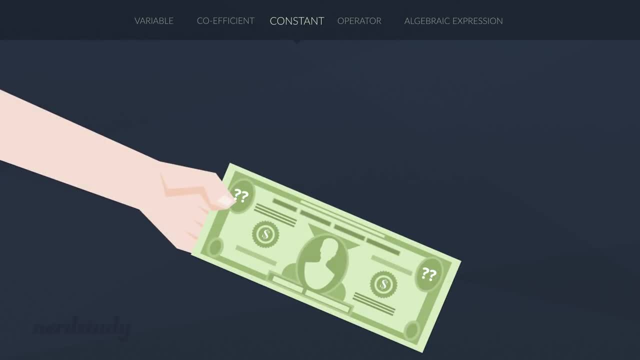 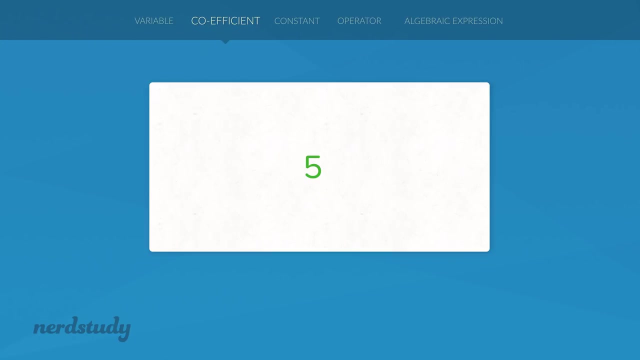 change. But when we're dealing with an amount that we don't know, that's when we use a variable, And of course the value can then vary. So to clarify: in this situation this number is a coefficient And in this situation this number is called a constant. 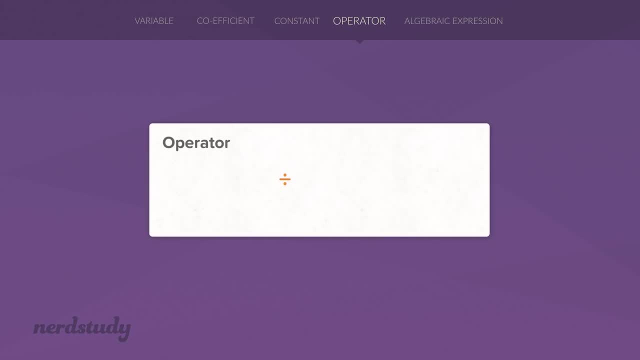 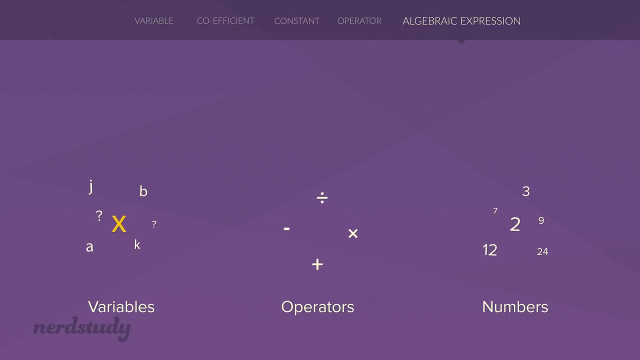 Next up is an operator, A division sign, a multiplication sign, an addition sign and a subtraction sign. These are all called operators. Now you might have seen variables, numbers and operators come together to form math phrases such as 3x plus 2.. 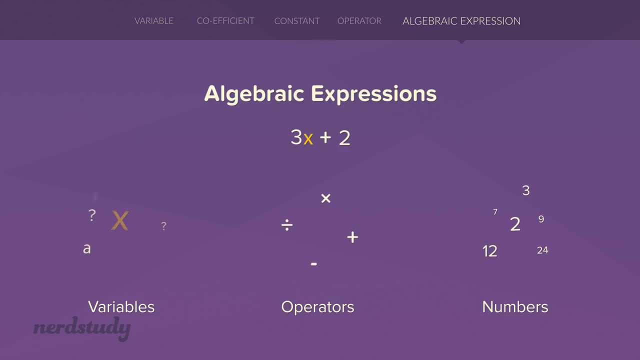 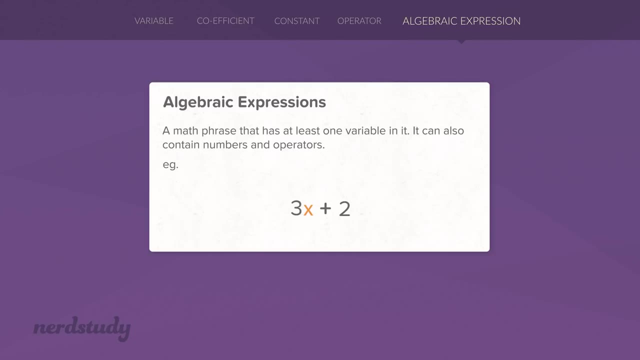 These are called algebraic expressions. An algebraic expression is a math phrase that has at least one variable in it, and it can also contain numbers and operators. Now, because it has a variable in it, its final value can vary. So let's take a look at some of the different. 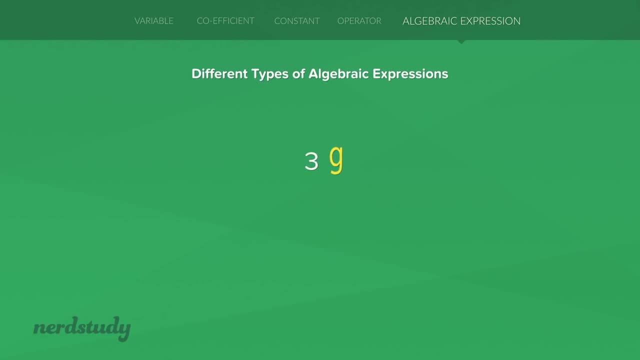 types of algebraic expressions. As we can see, this algebraic expression has a coefficient and a variable. This one has a division between a number and a variable, And this one has a constant being added with a coefficient multiplied by a variable. Lastly, this one is just the variable by itself. 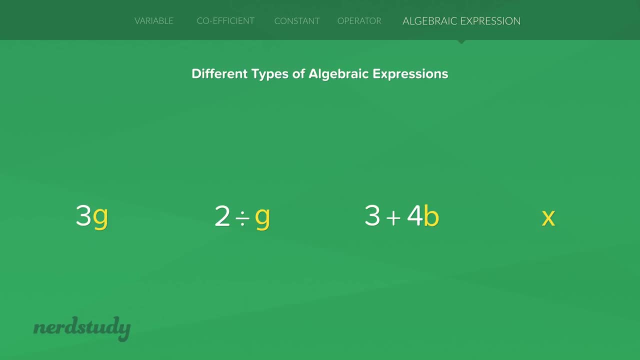 Of course, these algebraic expressions could also be expressed with English phrases. The first one is the equivalent of the English expression 3 multiplied by a number. This one is the equivalent of the English expression 3 multiplied by a number, or another way to say this. 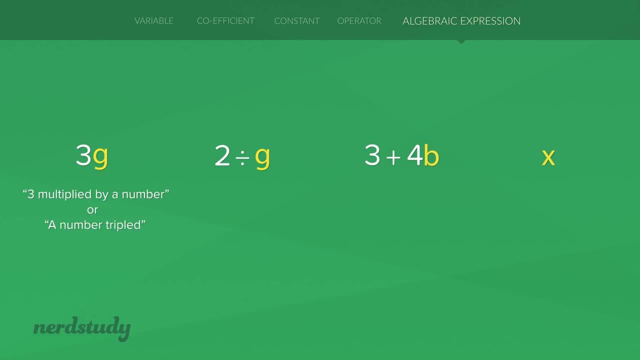 would be a number tripled. So if you were asked to mathematically express this, then you should be able to get this: And for the second one, 2 divided by a number. For the third one, we can say 3, more than the quadruple of a number. And lastly, 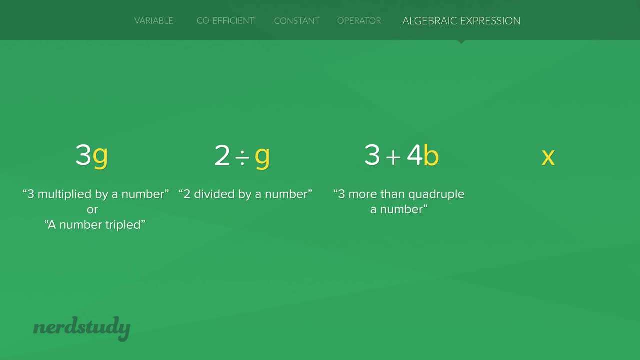 this one is the easiest to express in English. It would just be a number or an unknown number. So what if I told you to write down an algebraic expression for the sum of a number and 5. Then we can choose a letter of our choice and write x plus 5.. What if, instead, we said the sum of 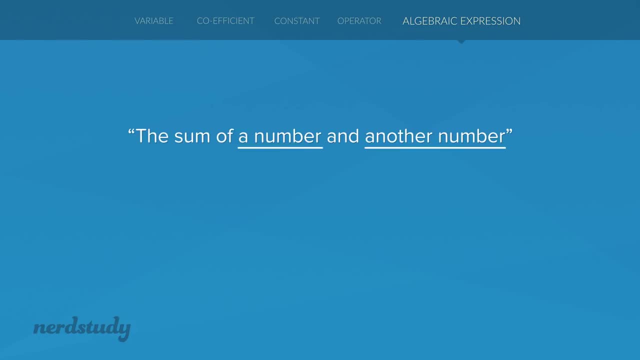 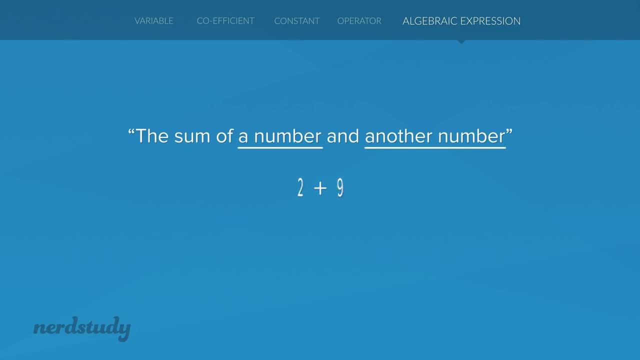 two unknown numbers might be different, or it might not be different. So in this case I'm going to choose x and y, and our expression will be x plus y. So again, notice here that we have two different variables. This means that the values of 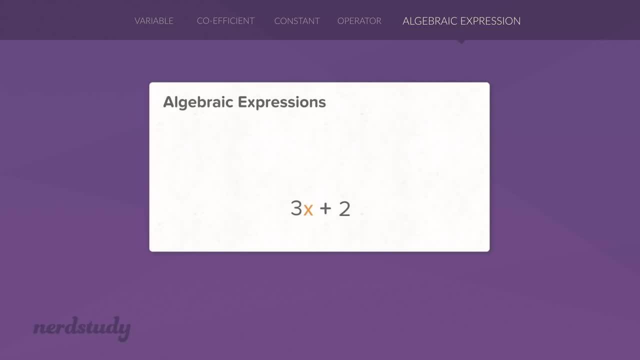 An algebraic expression is a math phrase that has at least one variable in it, and it can also contain numbers and operators. Now, because it has a variable in it, its final value can vary. So let's take a look at some of the different types of algebraic expressions. 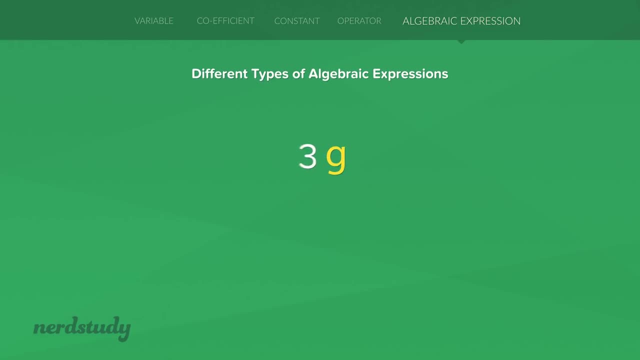 As we can see, this algebraic expression has a coefficient and a variable. This one has a division between a number and a variable, And this one has a constant being added with a coefficient multiplied by a variable. Lastly, this one is just the variable by itself. 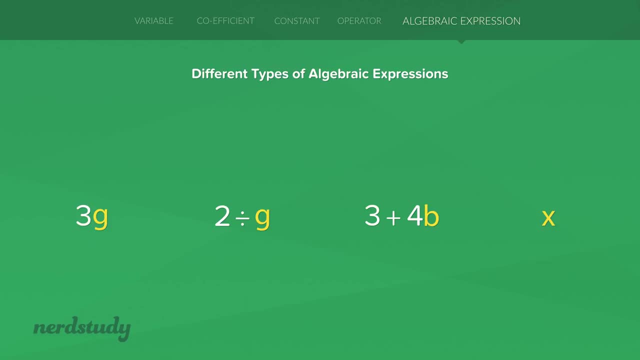 Of course, these algebraic expressions could also be expressed with English phrases. The first one is the equivalent of the English expression 3 multiplied by a number, Or another way to say this would be a number tripled. So if you were asked to mathematically express this, 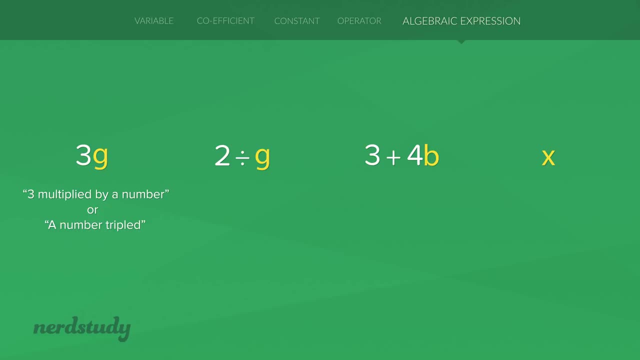 then you should be able to get this: And for the second one, 2 divided by a number. For the third one, we can say 3 more than the quadruple of a number, And lastly, 2.. It's not a singularity, It's basically a накles twin uppercase. 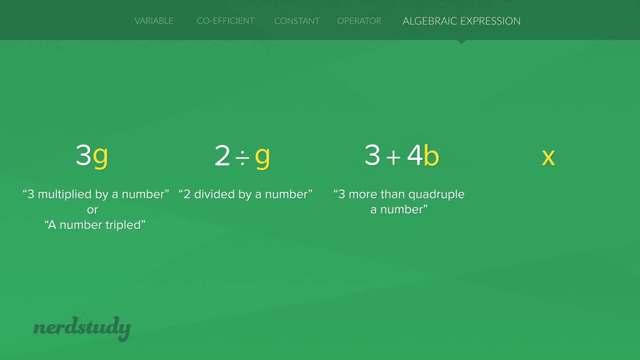 is the easiest to express in English. It would just be a number or an unknown number. So what if I told you to write down an algebraic expression for the sum of a number and 5?? Then we can choose a letter of our choice and write x plus 5.. 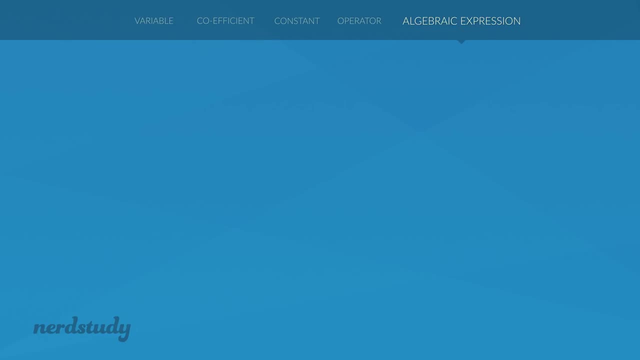 What if, instead, we said the sum of a number and another number? In this scenario, we should use two different variables, because we have here a number and another number. This means that the two unknown numbers might be different or it might not be different, So in this case, I'm going to choose.